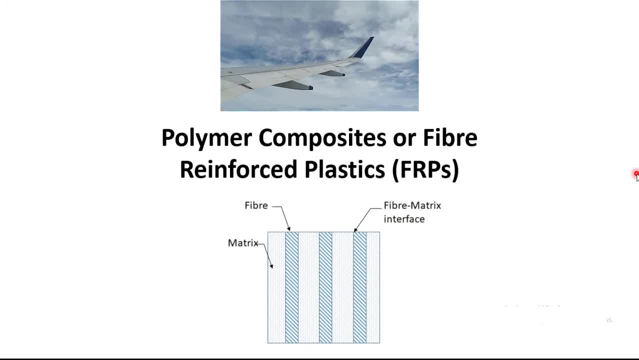 The matrix and the filler are chemically different and there is no chemical reaction between them, But they form good bonds. This interfacial bonding may be enhanced by some chemical or physical treatment of the fibers. Though the concept of composite material is very old, going back to the antiquity, the modern plastics-based composites were developed in the 1930s. 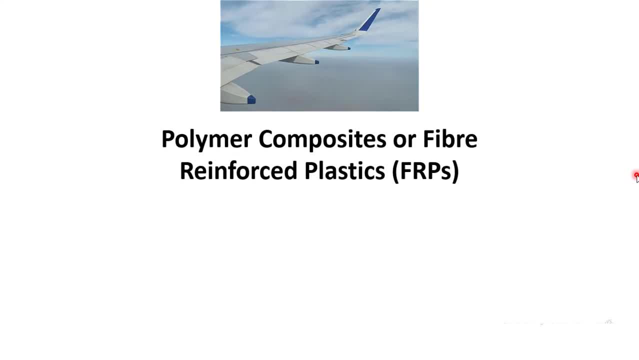 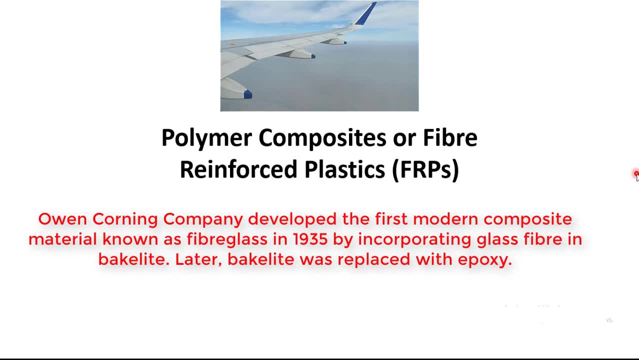 This class of material was originally developed by the company Owen Corning in the USA, and this type of composites are known as fiberglass. They contain chopped or continuous strands. The fiberglass is a material that is made of continuous strands of glass fiber with matrix of epoxy or other polymers. 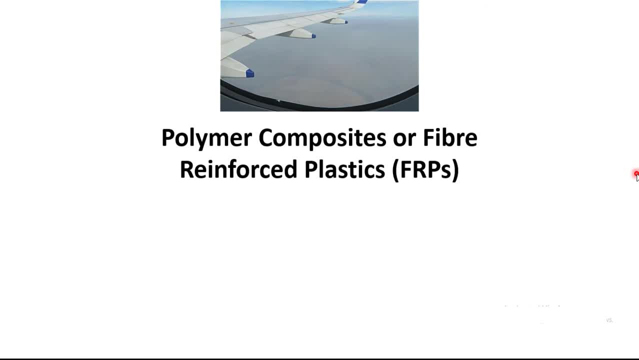 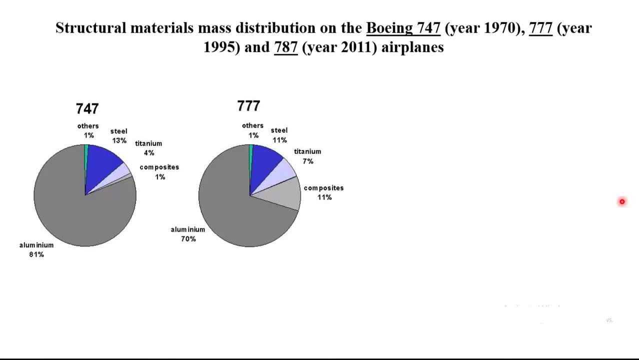 However, as of today, there are many types of fibers and matrix polymers used for advanced composites. The biggest impact of the use of advanced composites can be seen in the aircraft industry. Today, much of the efficiency and load bearing of aircraft can be credited to the use of carbon fiber epoxy composites. 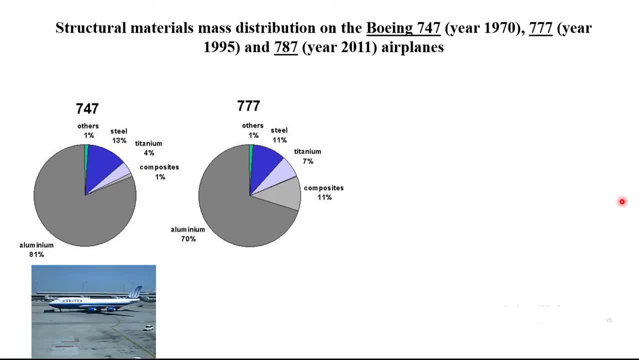 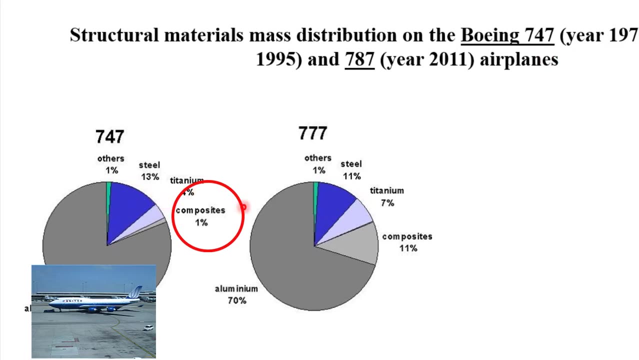 These are the lightest and strongest materials available In the passenger aircrafts were used from 1970s. For example, in Boeing 747, the jumbo jets, the percentage of composites used was 1%. This increased to 11% by weight in Boeing 777. 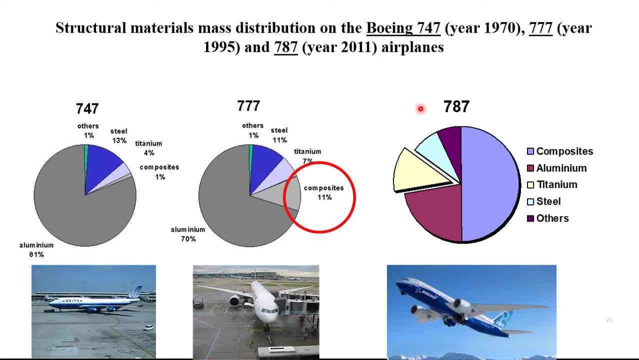 And or Boeing 787, the dreamliner. about 50% of material is by weight- is composite Carbon fiber epoxy composites are used. Carbon fiber epoxy composites are used as structural materials for the fuselage, wings, tail doors and much of the interior. 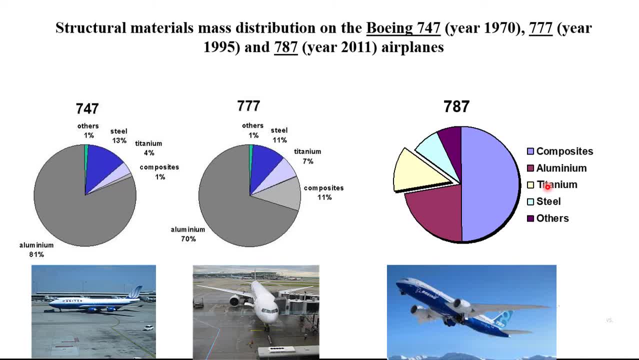 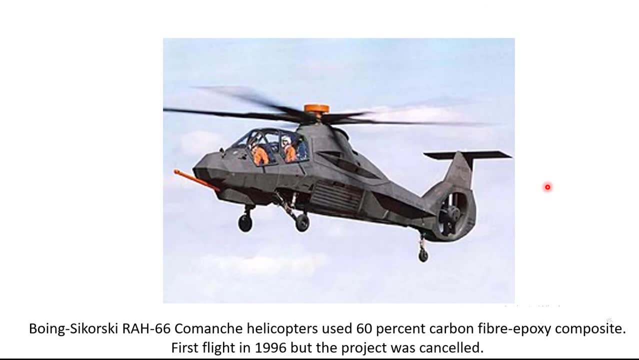 Lightweight composites enhance an aircraft's efficiency in load carrying capacity and huge advantage in fuel saving. In fact, the very first large-scale use of carbon fiber epoxy composite was the Boeing Sikorsky helicopter, in which 60% by weight was this composite. 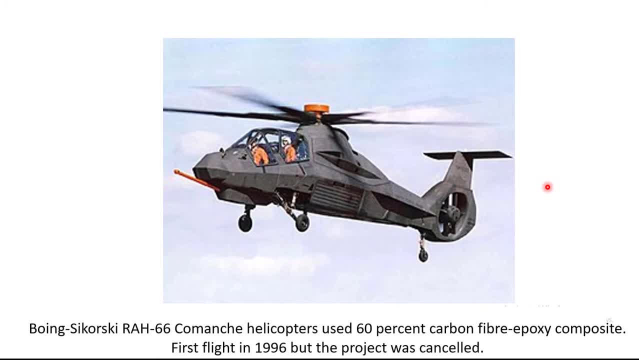 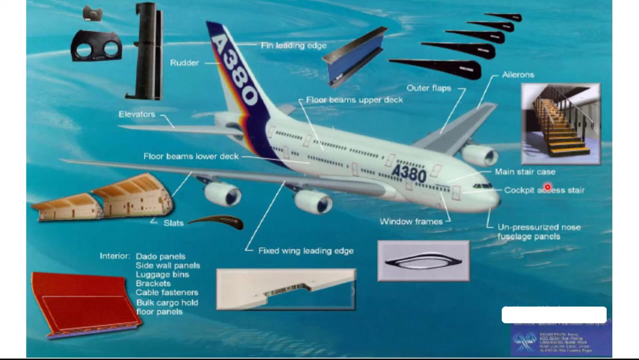 Started in 1991, this helicopter was designed as a stealth and attack helicopter. However, because of the long delay, budget overrun and the end of the Cold War, the helicopter project was terminated in 2004.. The Airbus A380 also uses fiber reinforced composites for many of its parts, though the fuselage is still of metallic type. 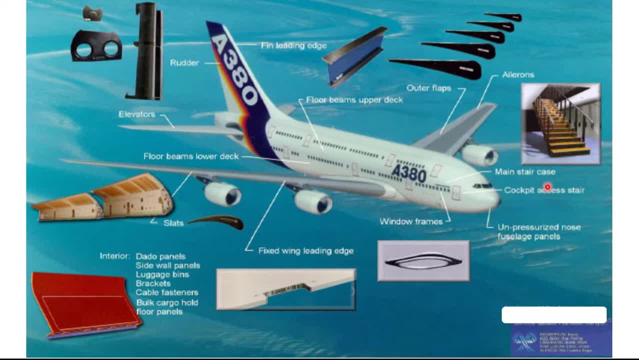 A380 uses carbon fiber reinforced plastics for wing ribs, upper deck, floor beams, center wing box, landing gear and the fuselage. This��r upgrade is still 누가ição esto ótima sucederá. Center wing box, landing gear, doors, unpressurized fuselage, vertical and horizontal tail, plain tail cone, engine cowlings, flap track panel and much of the interiors. 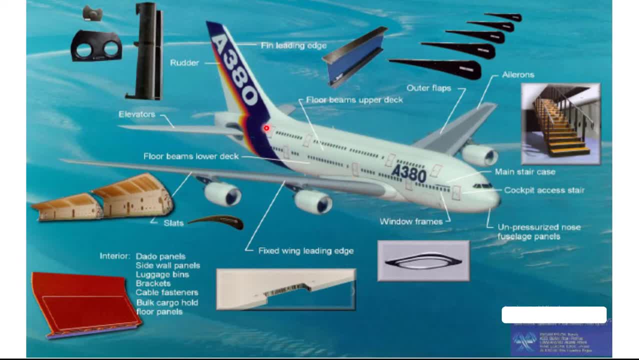 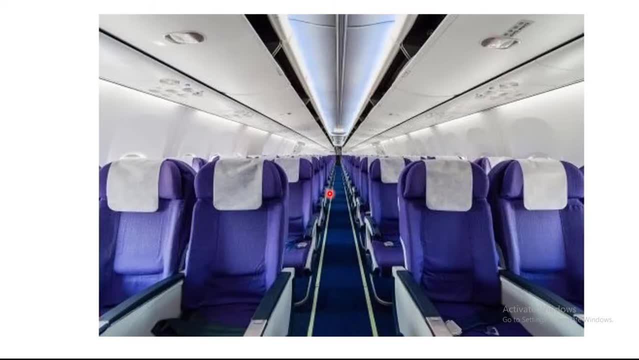 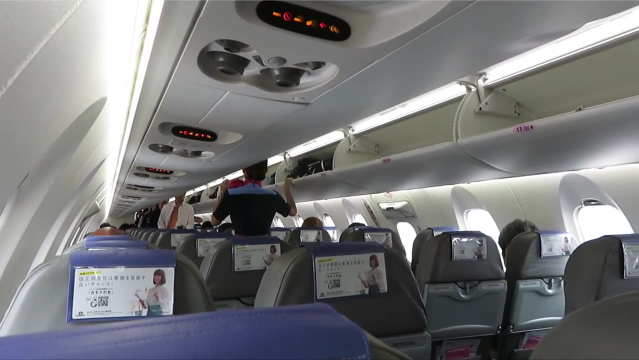 ング, wingbox, landing gear, doors, unextretifficient fus oggivo vertical and horizontal tail, plane tail con engine cowlings, flap track panel and much of the interiors. look inside of any airplane and you will find the interior is mostly plastics or composites. 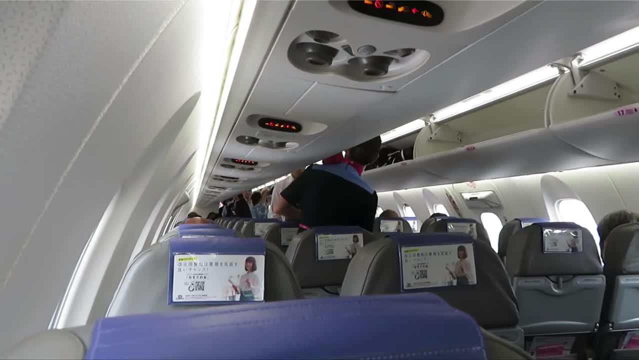 Look inside of any airplane and you will find the interior is mostly plastics or composites. This reduces the weight of the plane and hence adds to the fuel efficiency. 기� accounted as 단속 peut 파 opportunities to при Schluss användan 돼 emptiness. Все omitting is the weight of the plane and hence adds to the fuel efficiency. 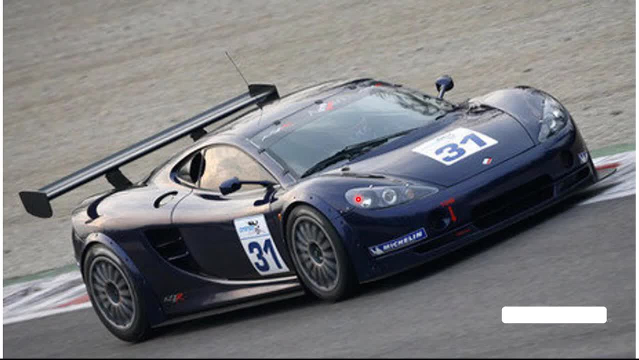 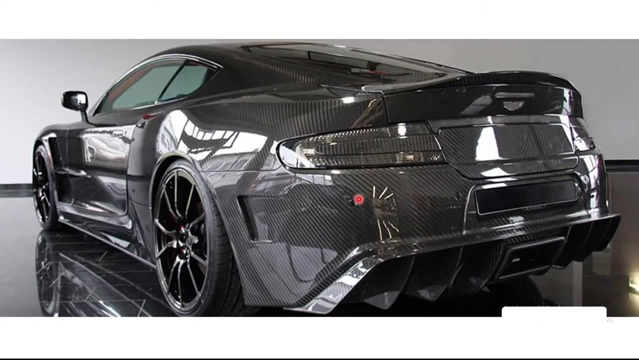 FRPs are already used in many sports and high engines. in many sports and high-end cars, Full body is made with carbon fiber epoxy composites. They save weight without compromising on strength and safety. Many years ago I had come across an accident site where a sports car had collided. 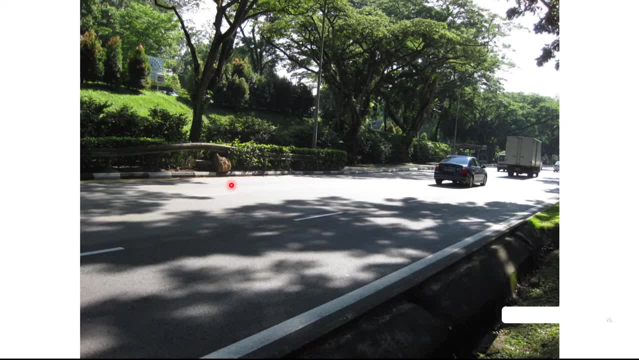 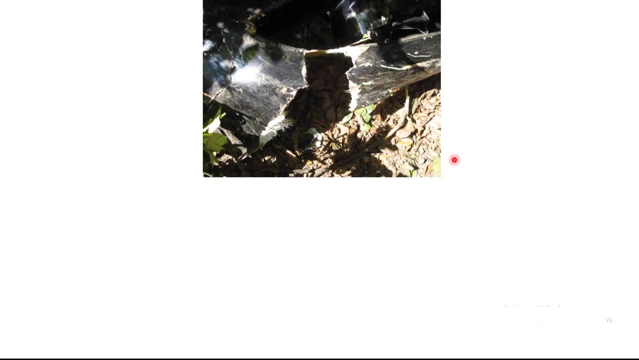 with the guardrails on the roadside. The car had composite body and I could find many broken pieces as far as about 30 meters from the accident site. The failure of these composites is not of ductile type, but it has huge amount of toughness, due to the different failure mechanism of composite materials, than 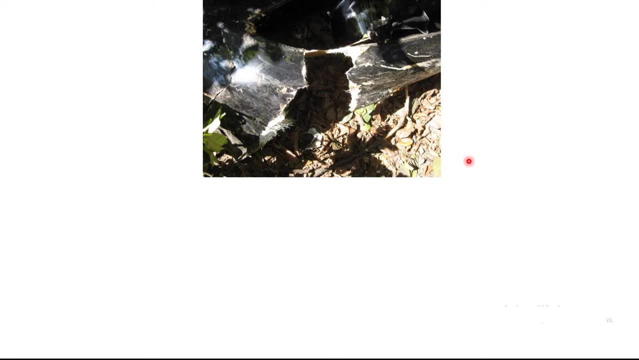 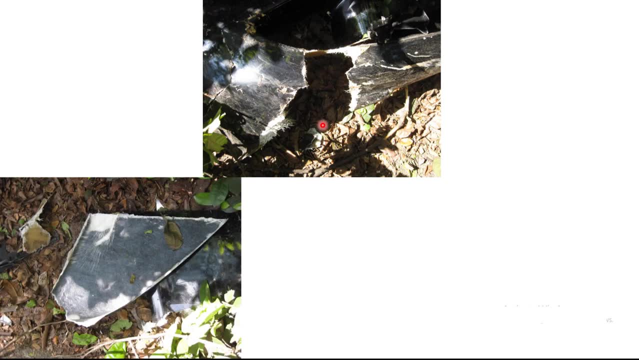 that of the ductile materials. The broken pieces appear to be made of hybrid carbon and glass fiber with epoxy as the matrix. These pieces break in a very characteristic brittle type of fracture. However, before they fracture, they absorb much of the energy and therefore they are very tough materials. 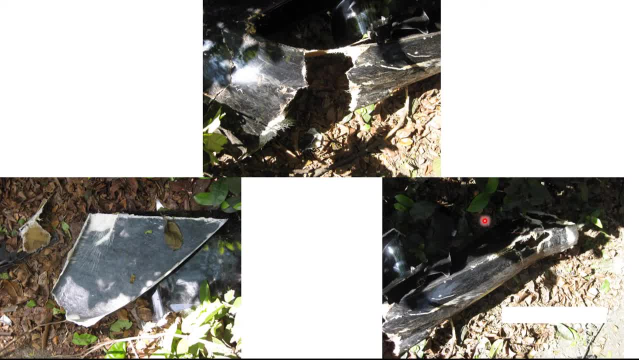 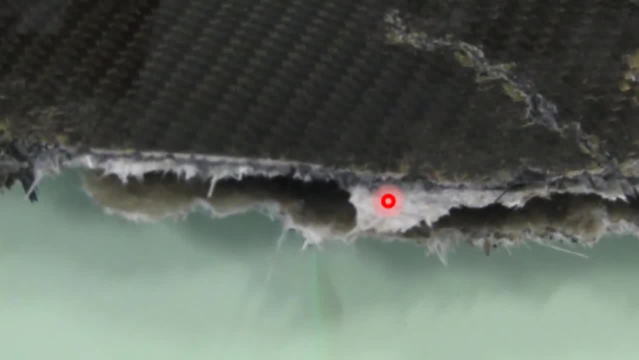 Here also we can see that the material has broken without much of ductility. In this piece we can see the inside of the composite material. So it appears to be a mixture of carbon fiber and glass fiber with epoxy as the matrix. So the white 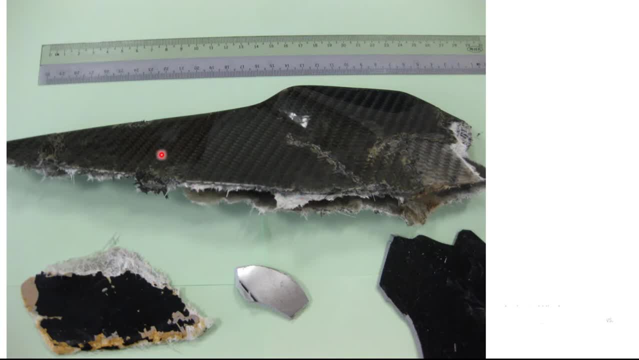 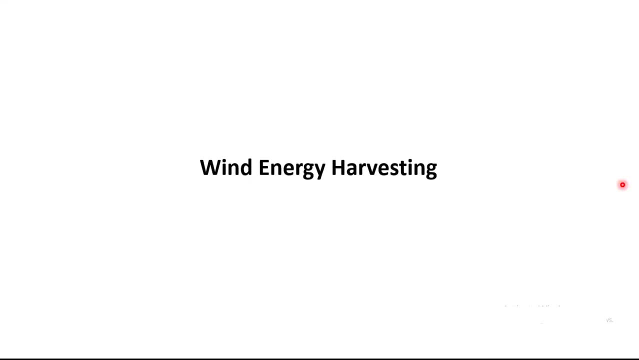 part is glass fiber, the black part is carbon fiber and epoxy is used as the matrix. Energy sector is also utilizing composites in a big way. As we are making machines bigger, lightness will increase and the material will be more durable. This is the usual thing which is being done on the planes with the same 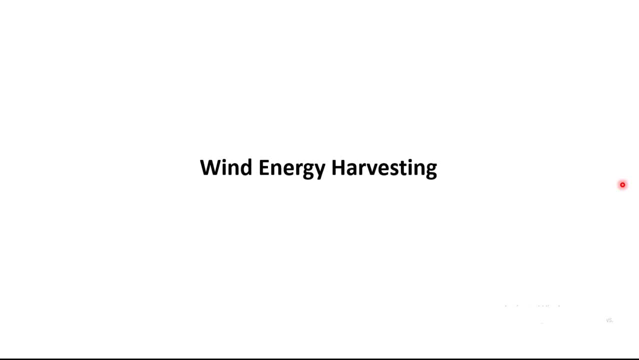 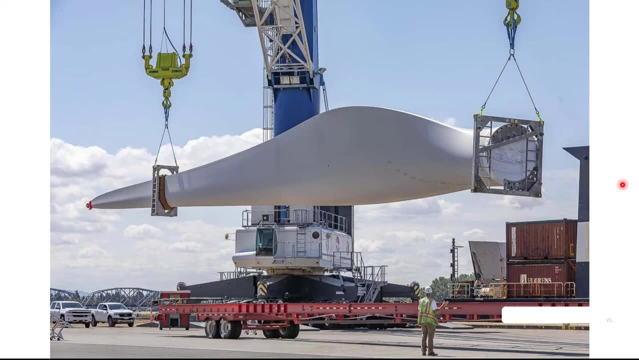 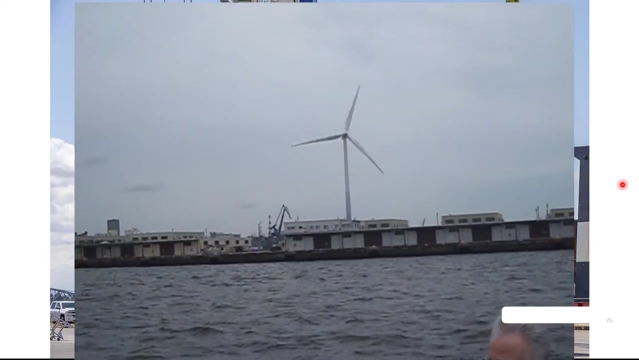 material, as we are using a lot of components. Here we can see the process of the same block as the main block. After the process the lightness will increase in the plastic material and as the metal gets larger it will become more durable. 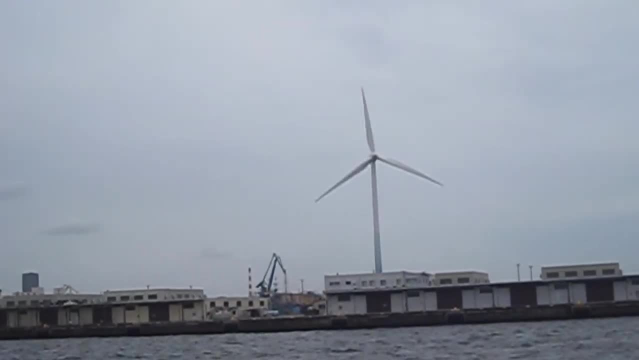 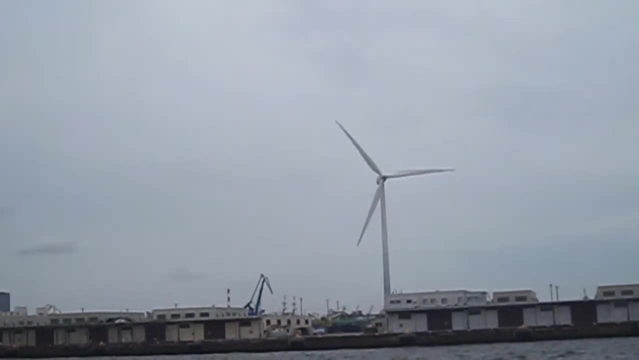 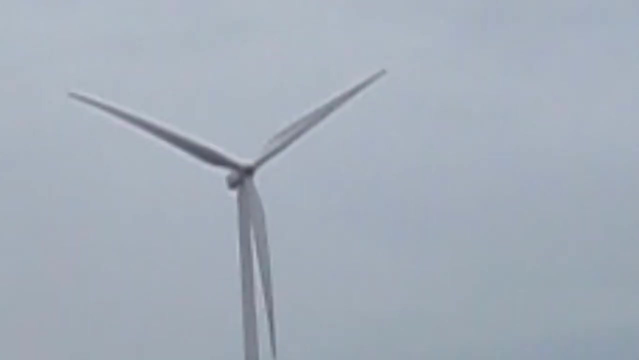 The solid metal will become more are as light as possible, but they also must be strong against wind power. they should be tough against impact loading such as strong wind, and must withstand all kinds of weathers: cold, heat, rain, sea environment, etc. carbon fiber and glass fiber are used with epoxy polymer to make such 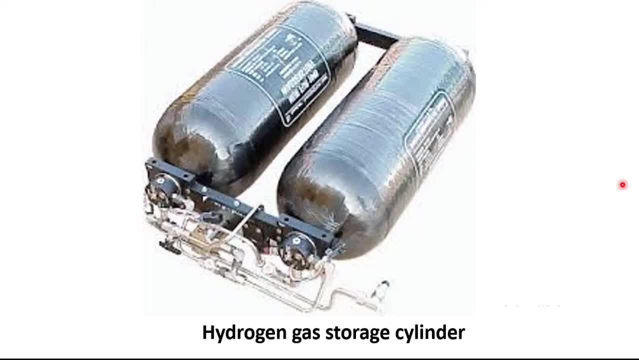 huge mechanical items. the other energy sector that urgently needs frps is the hydrogen gas based energy production. one of the challenges in this field is the storage of h2 gas, which is quite damaging for metals such as steel because of hydrogen embrittlement- also for any mobile energy. 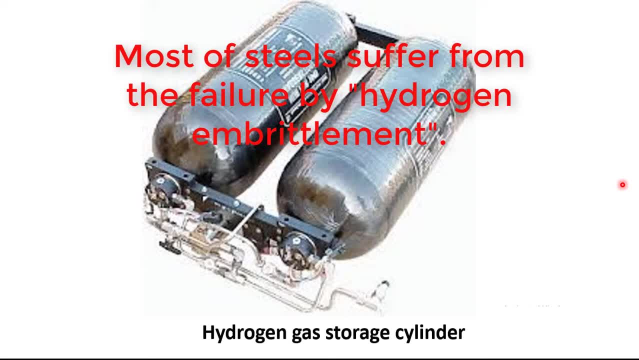 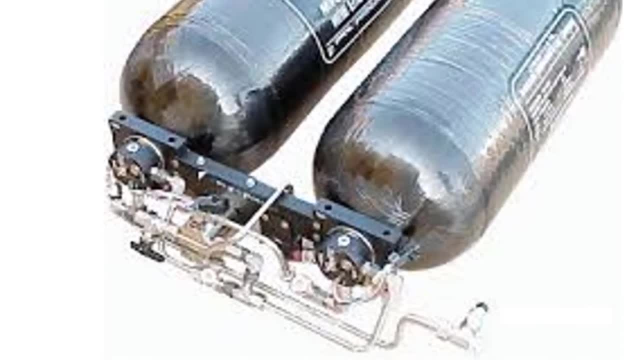 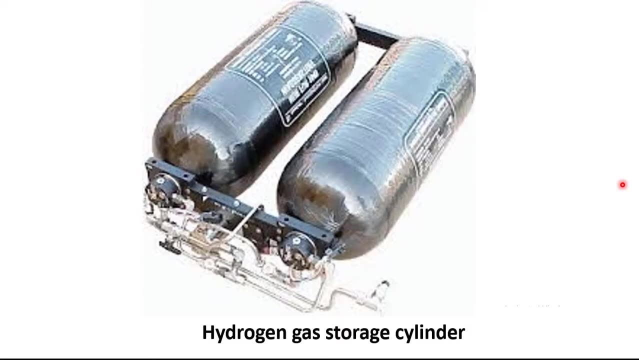 solution, such as for automotive application, it is necessary that the storage tank is very light, not a bulky steel cylinder. this is solved by having frps as the materials for hydrogen storage tank or cylinders with extremely high strength and toughness. a cylinder made of frps is able to store the gas at very high pressure, but with safety. 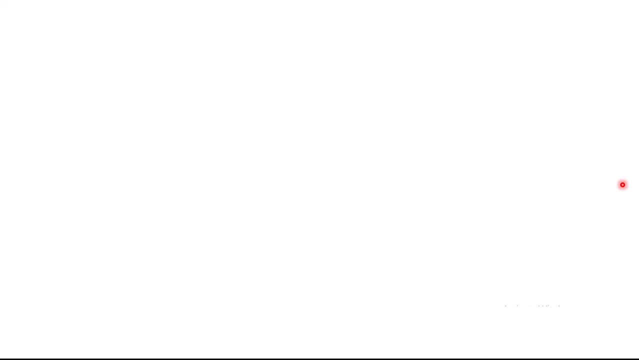 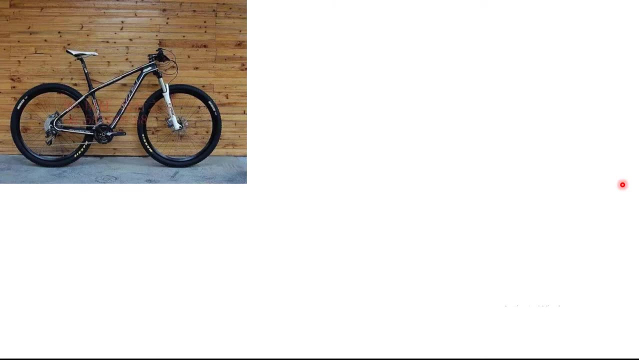 force have in general benefited immensely from advanced materials such as frps, for example. a racing bicycle can be made very light by using carbon fiber epoxy composites instead of steel or aluminium frames. a lighter bicycle will be easier to ride in a race, rowing or any kind of 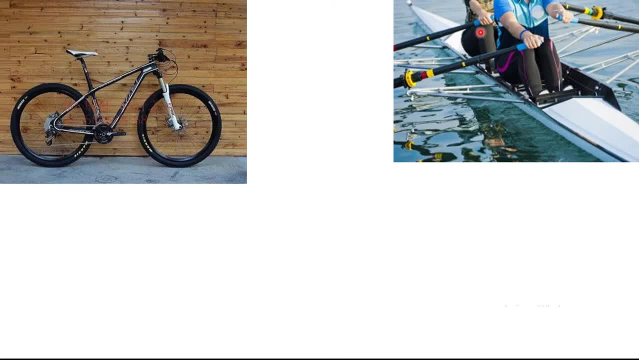 water sport depends on materials that are strong, stiff and light. often glass, fiber or carbon fiber based plastic composites are used for making the boards, holes and any kind of floating boards, etc. today, all tennis rackets are made of glass, carbon or aramid fiber based plastic composites. they are lighter, with optimum strength and its stiffness. 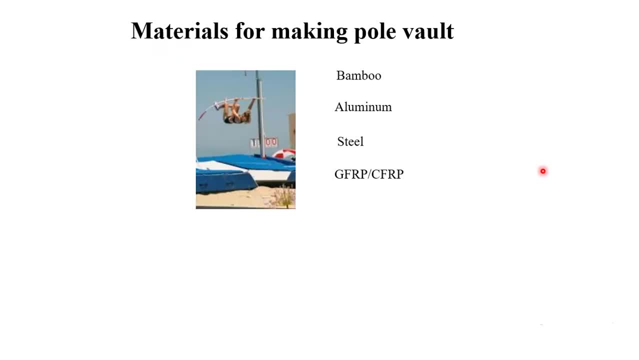 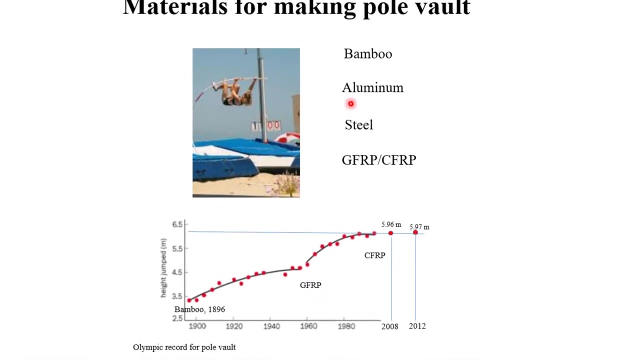 let us look at materials for making pole vault. pole vault uses materials such as bamboo, aluminium, steel, gfrp. that means glass fiber. carbon fiber based plastic composites are used for making the glass fiber reinforced plastics and carbon fiber reinforced plastics. very early days, bamboo was used as the material. it was followed by aluminium and then steel, and we can see how this sport has. 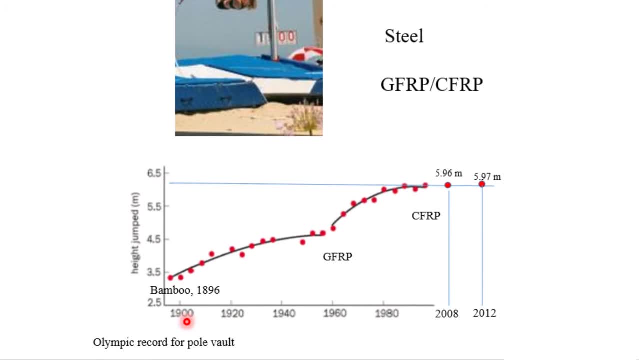 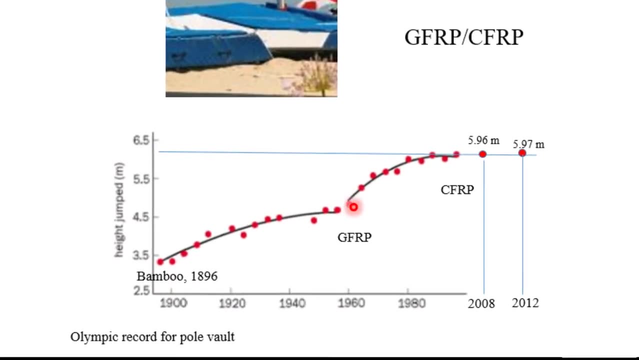 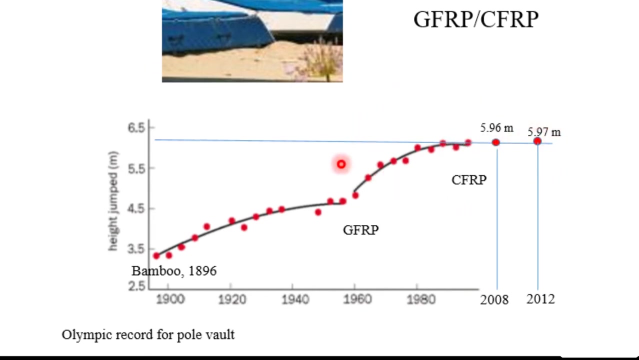 benefited with advanced materials. the height jumped- and here we have the years when the olympic was held. we can see that as the materials have been changed, the height jumped record has increased tremendously, and this is much to do with the new materials in addition to the new techniques of the sports. so we can say that sports performance 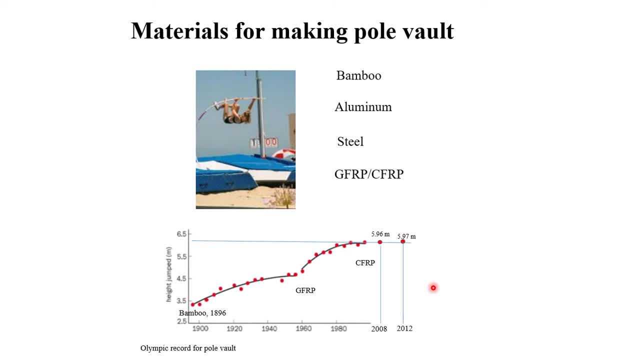 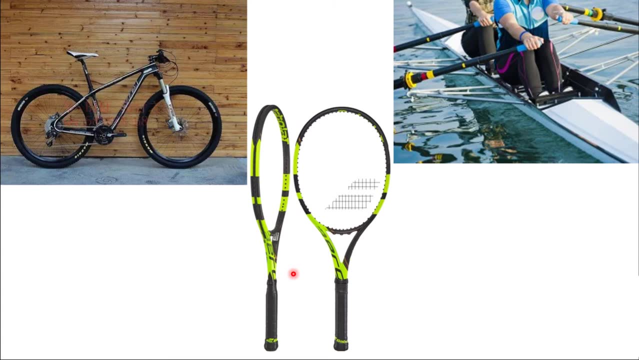 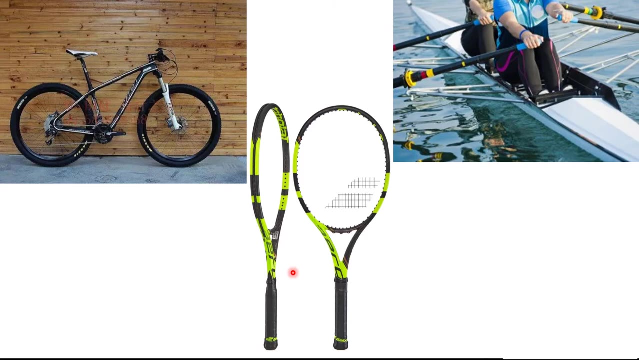 is hugely benefiting from new advanced materials. composites are considered advanced materials when we use the component materials such as carbon glass or aramid fiber and matrices which are thermoset or thermoplastic polymers. but if you look around, you will find many old things. 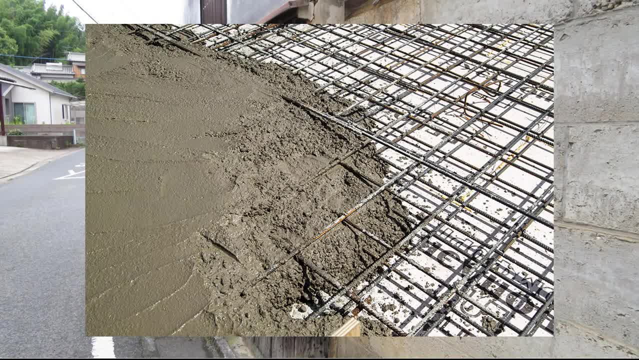 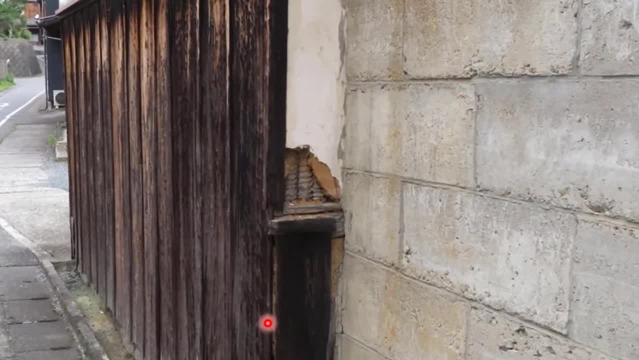 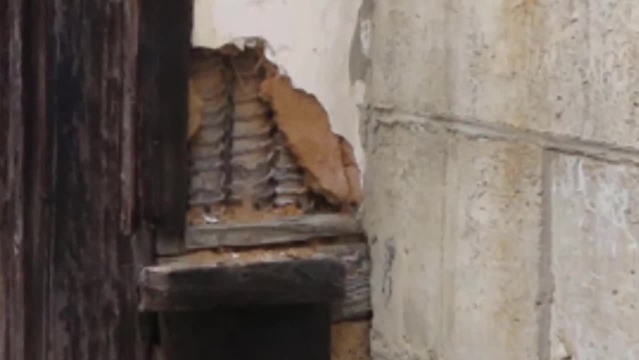 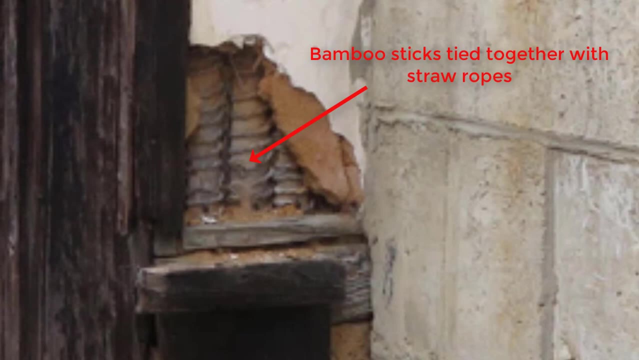 that use these concepts. construction industry uses steel reinforcement materials such as concrete, which are composites. in japan, i looked at some old wooden houses such as this one, this damaged area. you can see what is inside. bamboo sticks have been joined together with the help of straw ropes which were then covered with clay. here, the bamboo sticks act. 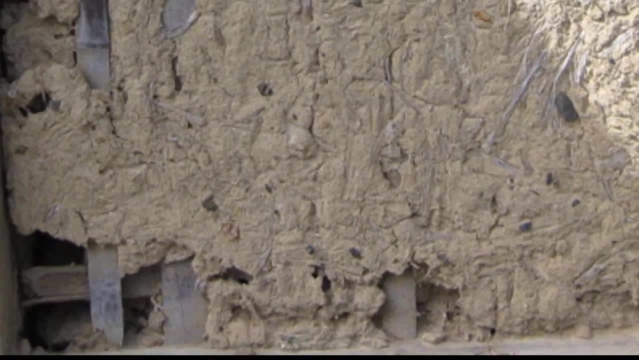 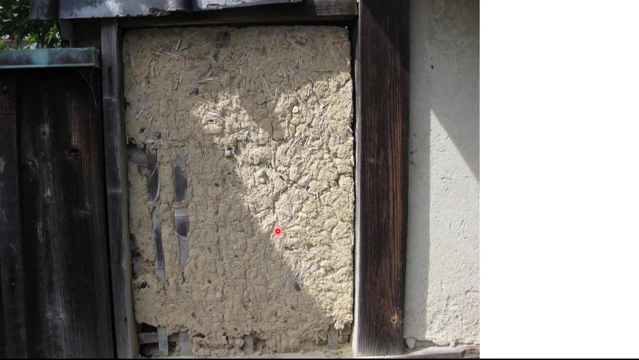 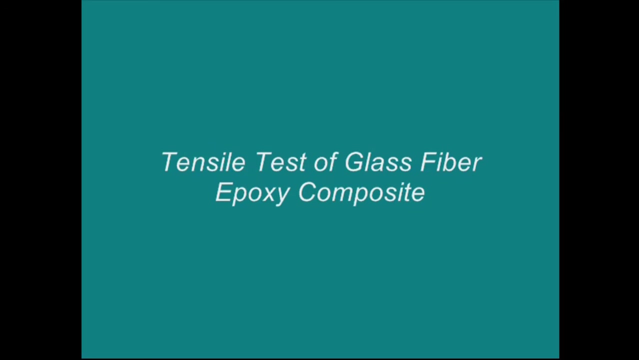 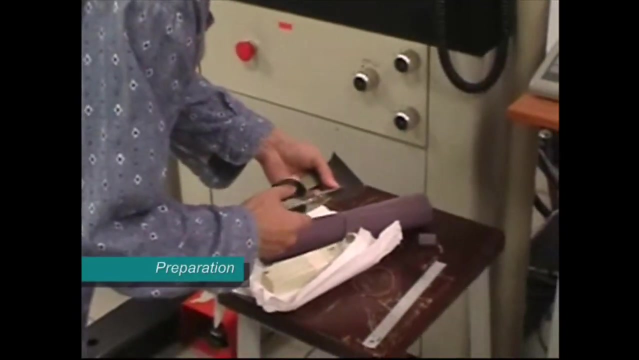 as the fiber and the clay as the matrix. some straw has been used in the clay for strengthening purpose, many ancient civilizations making mud bricks for the same purpose of lightness and strength. before i summarize this video, let me show you two experiments which we conducted on glass fiber. 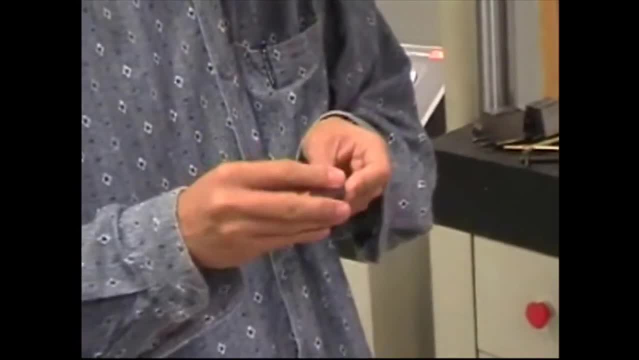 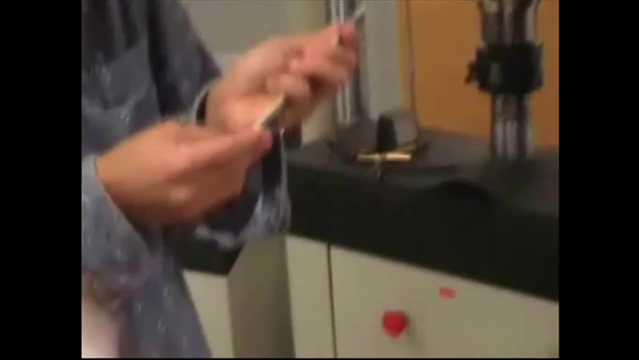 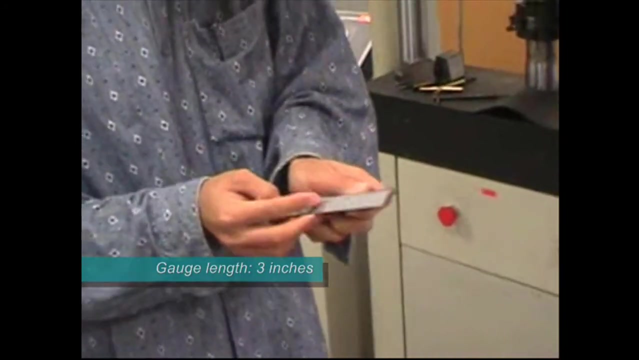 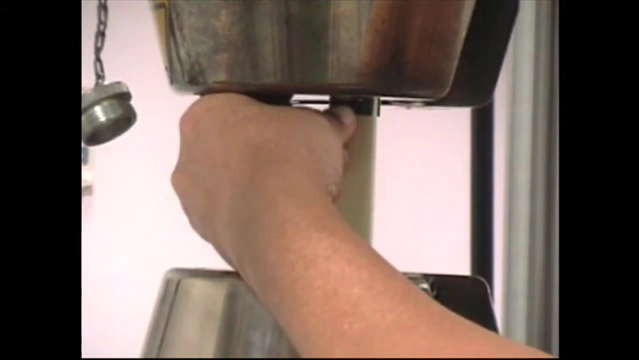 reinforced epoxy composite. so this experiment is on the tensile experiment on this composite. so there is a astm standard for testing polymer composites so you have to follow the astm standard. for specimen size, this specimen has a width of 25 millimeter and thickness of three millimeter. 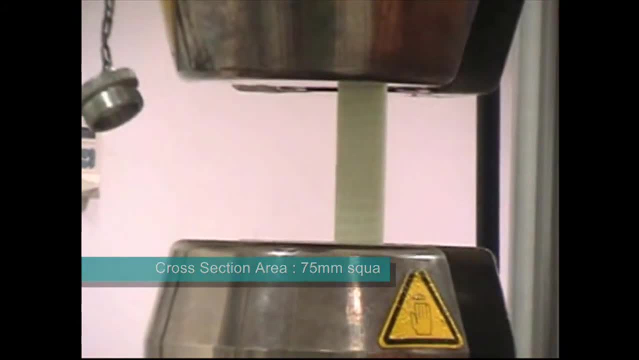 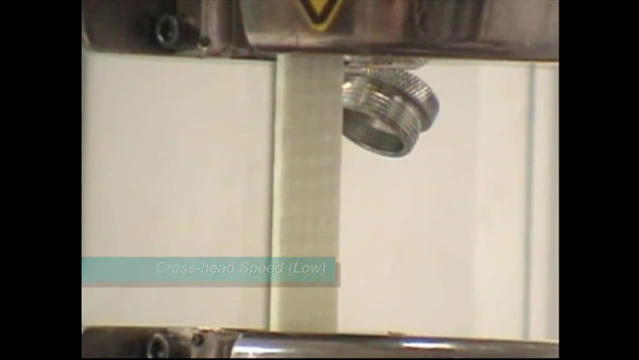 cross sectional area is 75 in square. so now we will keep the crosshead speed of the instrument and we will reduce the machine as low, which is 0.5 mm per minute. so after the experiment, you can see the failure has happened. actor near the one of the edge. 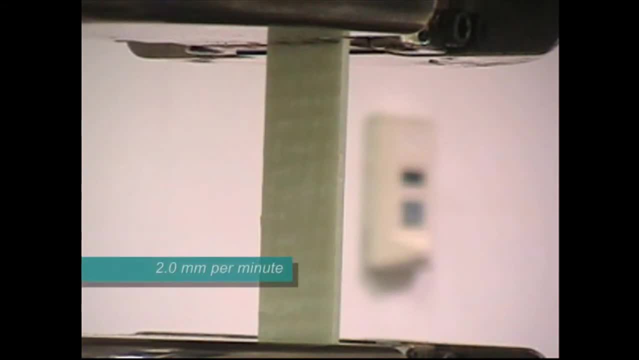 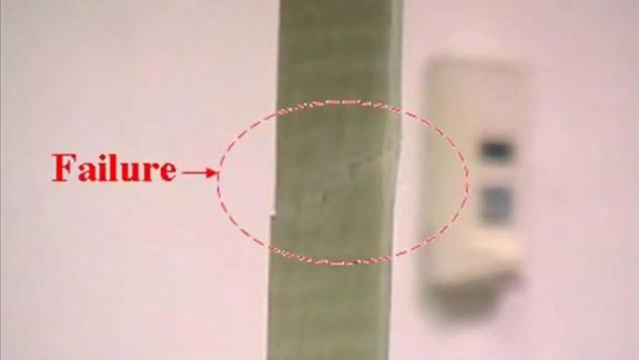 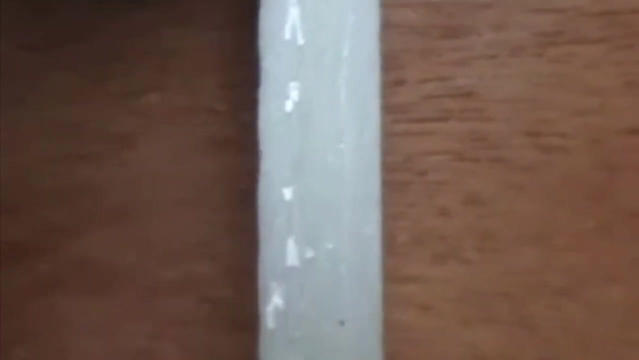 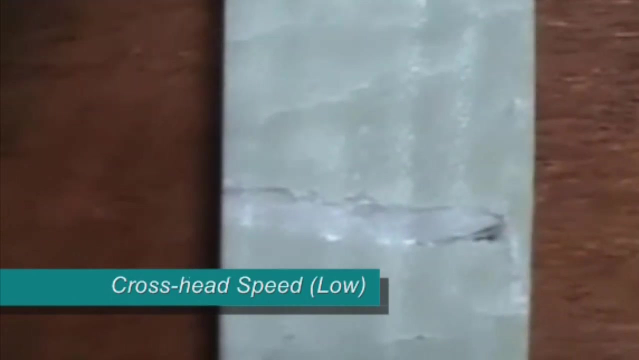 now we will conduct another experiment on the same specimen, so this time we will keep the crosshead speed of 2 mm per minute, and in this case the failure happened in the middle part. now this is the normal specimen that we have used and this shows the failed specimen, so you can see the delamination taking. 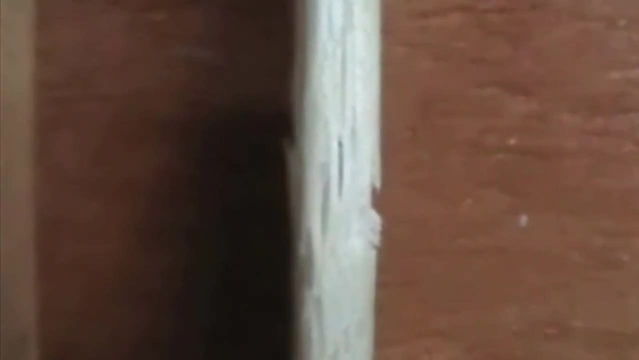 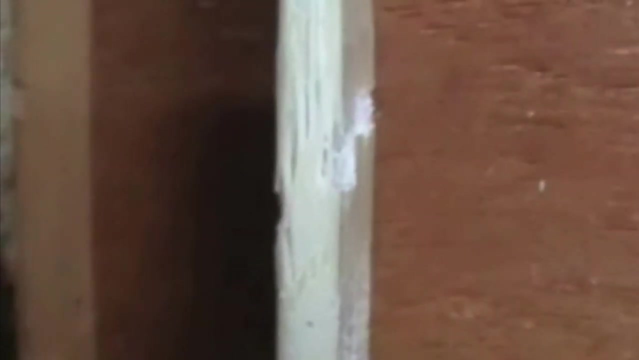 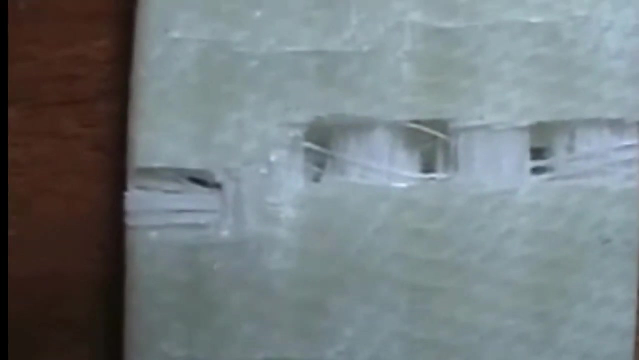 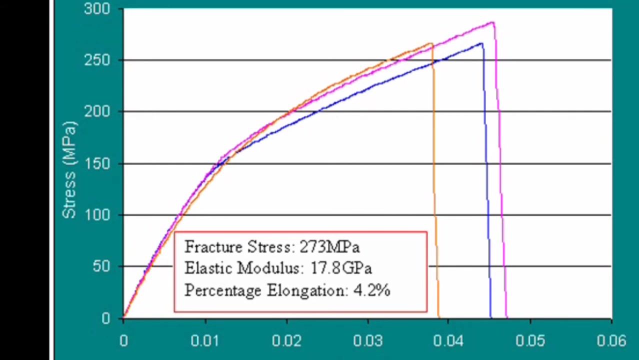 place and fracture of the glass fibers. so this is how a glass fiber reinforced composite would fail. so you can clearly see the glass fiber arrangement. so for the lower speed, lower crosshair speed of 0.5 mm per minute- the fracture strength was 273 mega Pascal. 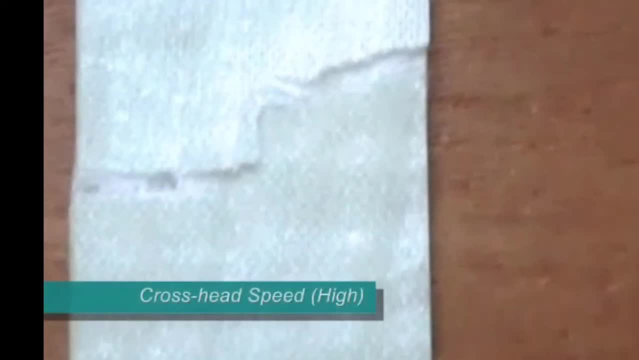 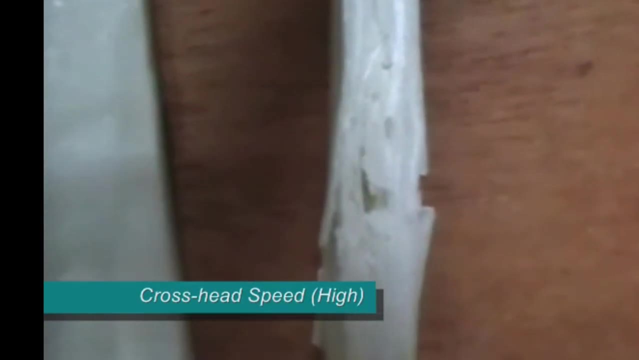 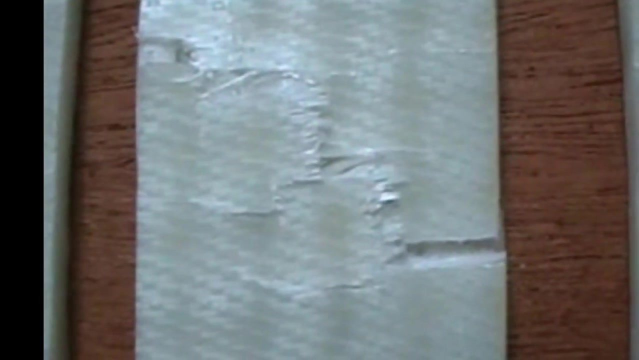 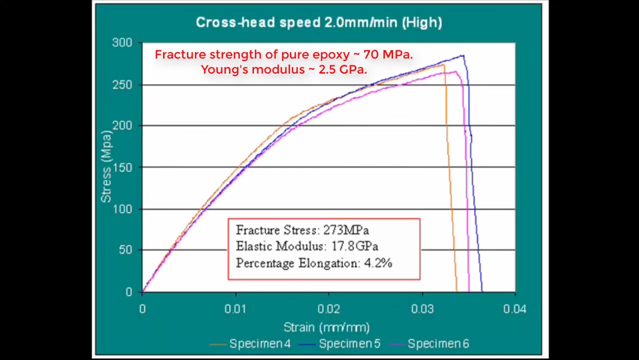 and elastic modulus was about 17.8 Giga Pascal. for the high crosshead speed specimen. again you can say: see that the failure mechanism is same, which is delamination between the glass fiber and the matrix and fracture of the glass fibers. for high crosshead speed test also, we see. 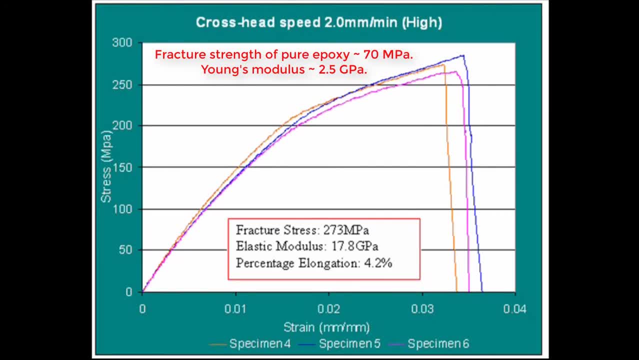 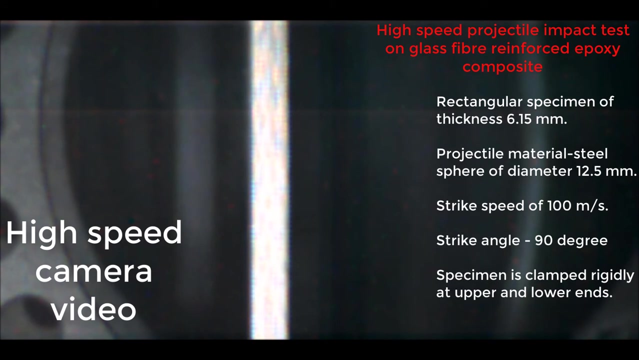 the fracture strength of 273 mega Pascal and the elastic modulus of 17.8 Giga Pascal. this compares with the pure epoxy value of fracture strength, 70 mega Pascal, and the young's modulus, 2.5 Giga Pascal. now I will show you another experiment in which we impact the glass fiber.